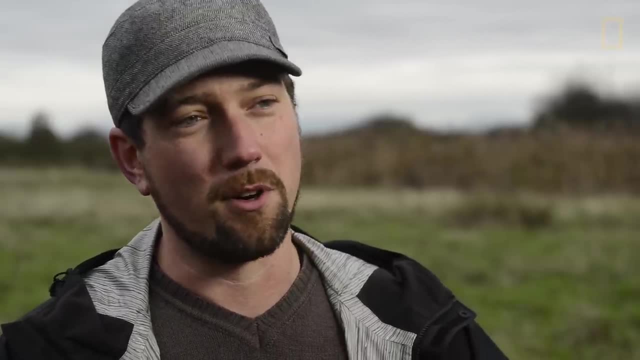 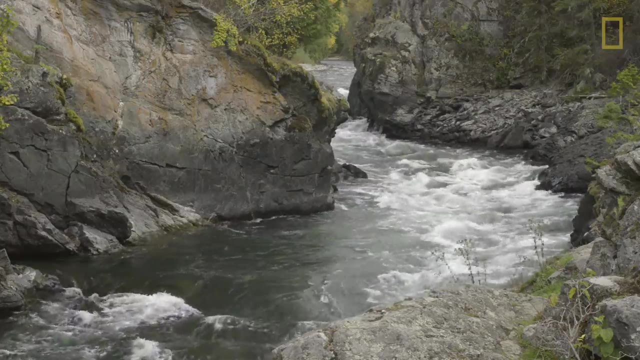 will go, you know, several hundred kilometers, over 1,000 kilometers, out to the mouth of the Fraser, then up along the coast, up into the Gulf of Alaska. So they're traveling several thousand kilometers in their lives and then they come back. 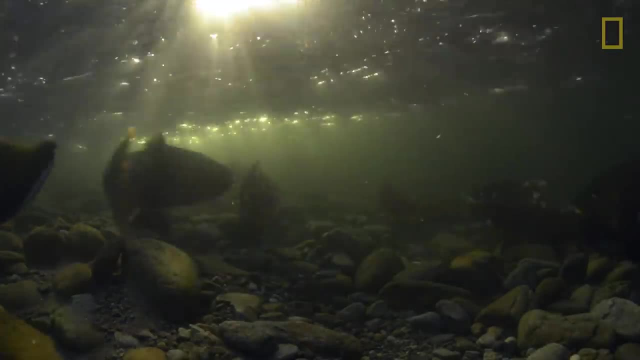 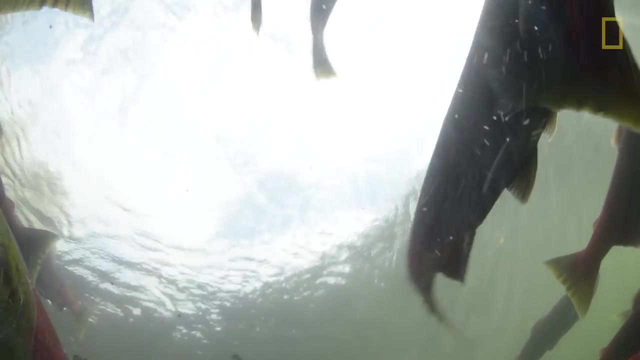 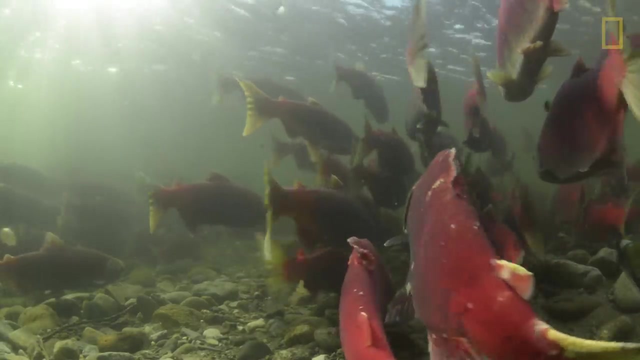 And so it's a massive migration Every four years. there's this massive population year, which is what we're in now, And then there's a shadow year- about half as many It's called a subdominant run- And then there's two years of really relative quiet. 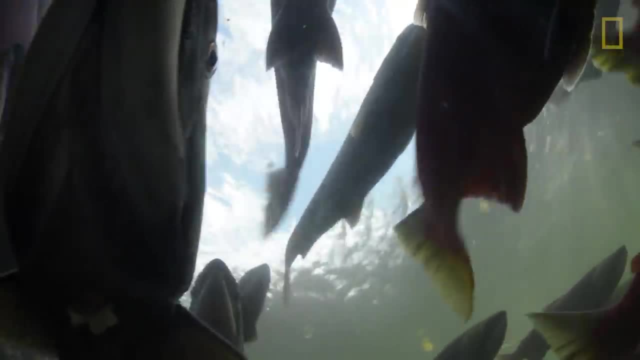 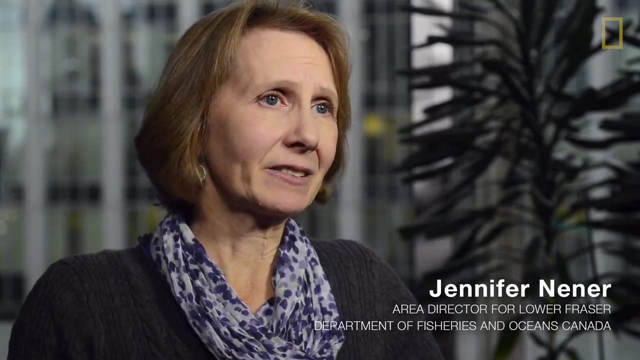 But generally speaking, it's evolved to be on this four-year cycle. So 2009 got a lot of attention because we had unexpectedly low returns. The total run size that year was about 1.5 million sockeye. coming back to the Fraser, 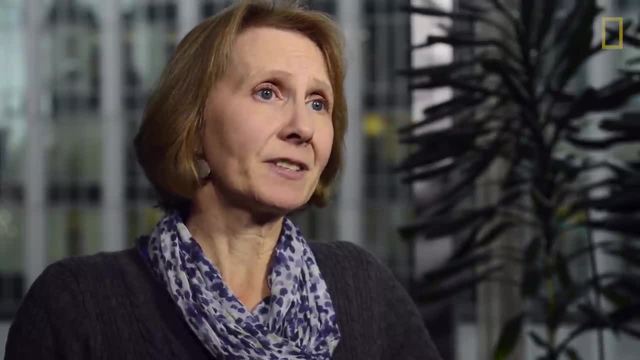 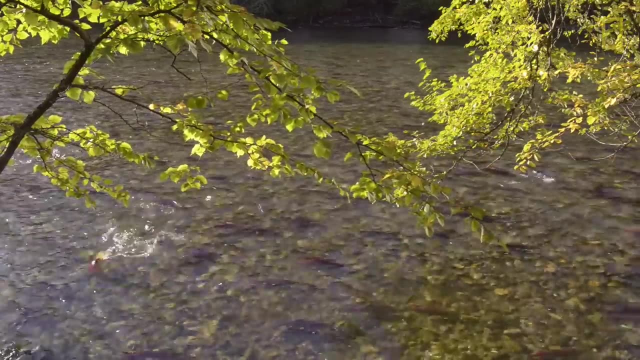 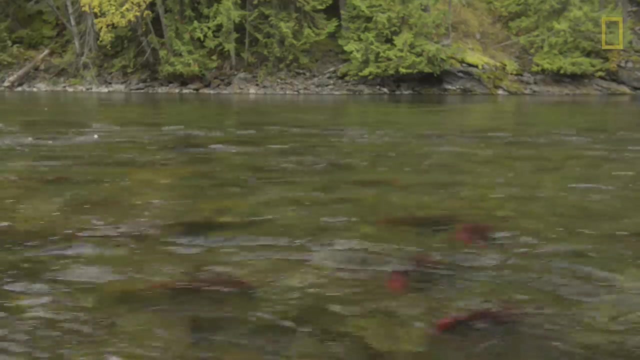 Four years previously. in addition to that, we had in the order of 7 million, So that was a significant decline and raised concerns. Where we're at today, obviously looking at about 19.6 or 19.8 million. coming back to the Fraser, 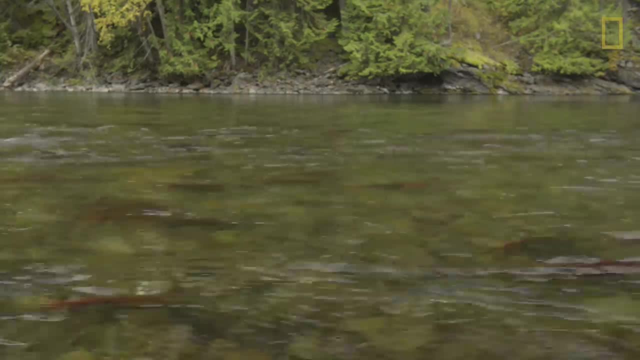 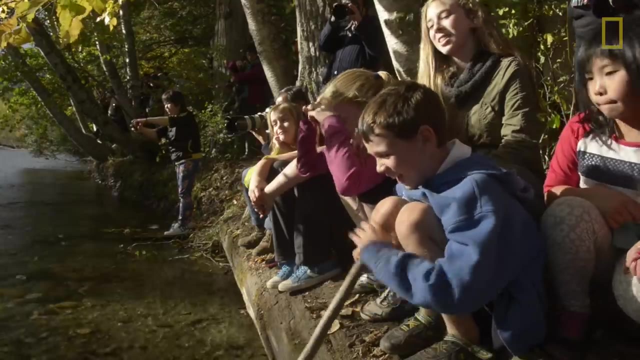 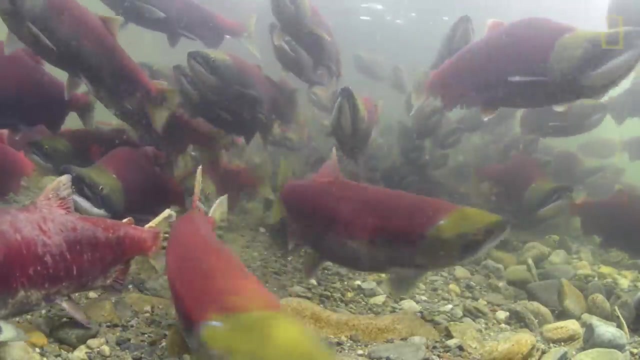 And I would say things are perhaps looking a little better for Fraser sockeye than people feared back in 2009.. We used to see returns like this on a regular basis over 100 years ago. One thing that we do know about Fraser sockeye: 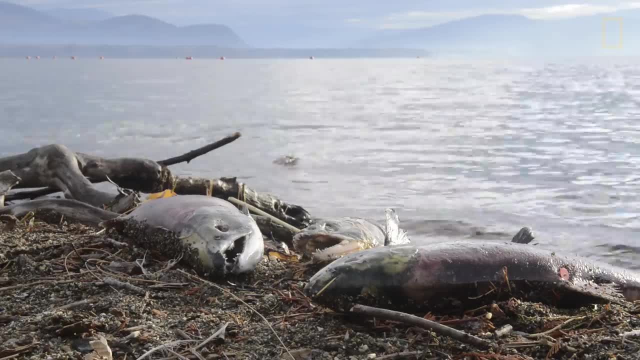 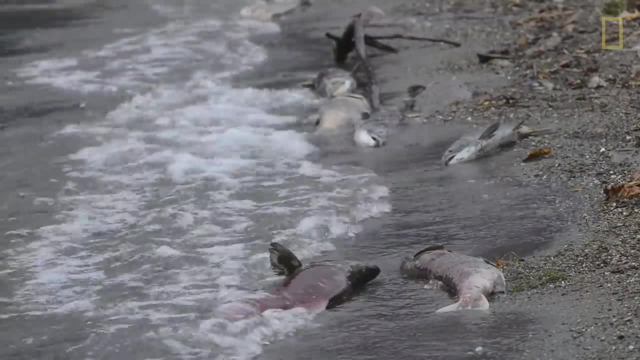 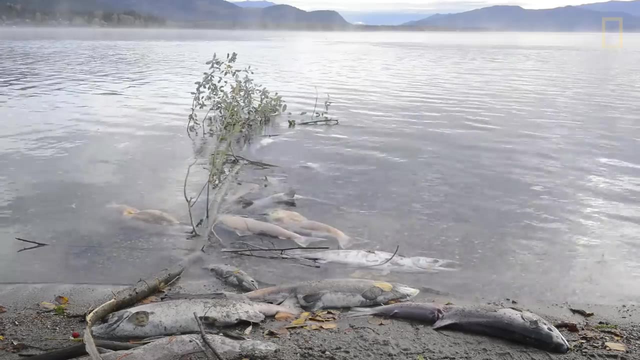 is they're being increasingly affected by climate change. We have in the Fraser River increasing high water temperatures in the summer And we have a number of weeks now in a lot of summers where the water temperatures reach a lethal threshold for salmon And that's going to increase as the climate warms. 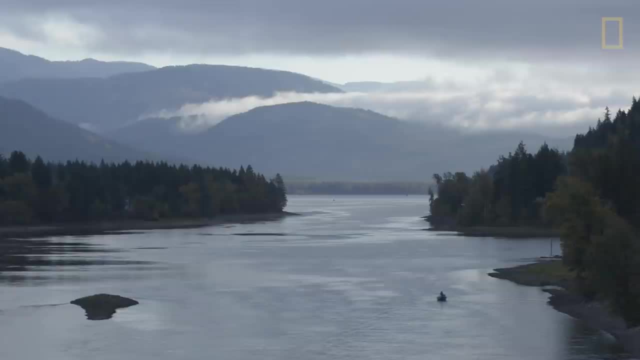 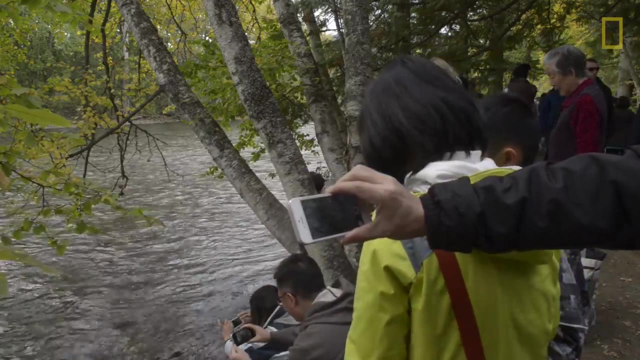 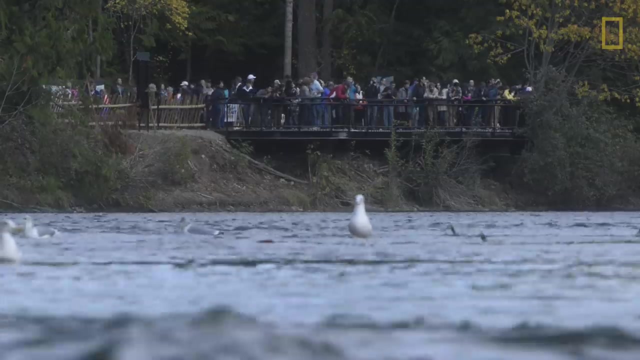 and as the river system increasingly changes. as a result of that, We have this abundant planet that we all share, And when you look at the cosmos and the universes around us, it's an anomaly. It's something so unique that has come together. 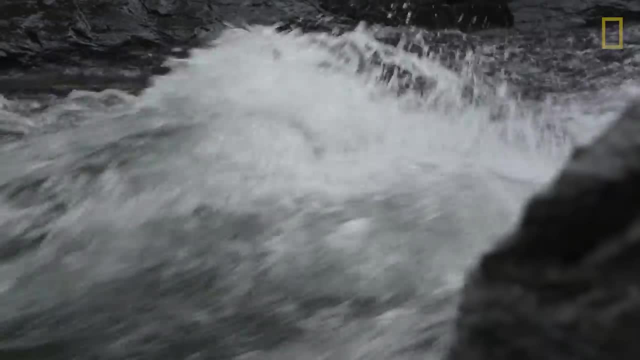 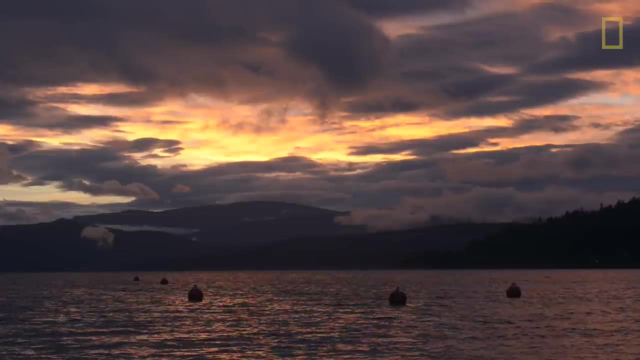 from so many thousands of potential disastrous conditions And we have a responsibility to care for it. We have a responsibility to be a part of it And we have a responsibility to embrace it. Embrace what it teaches us, And I think when we do that,